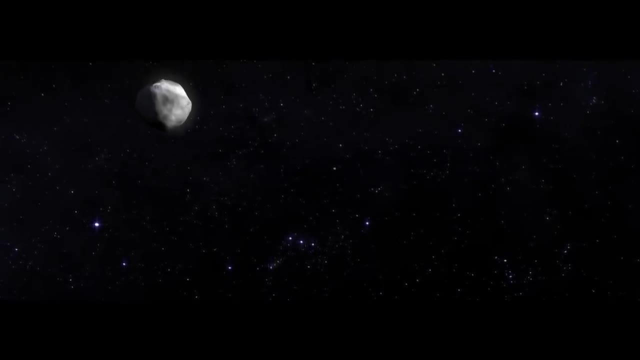 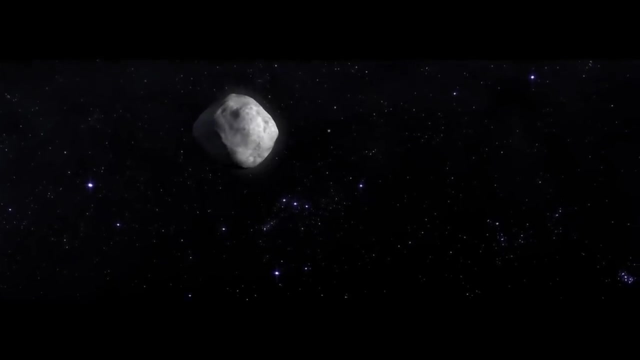 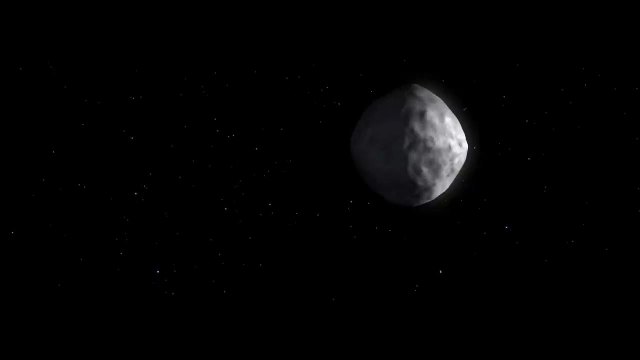 but deep questions remain. To answer those questions, astronomers are preparing to visit someplace very small, Asteroid, Bennu, A lump of rock and organic material, the early building blocks of the Solar System Of Earth Of us. Bennu is a time capsule. 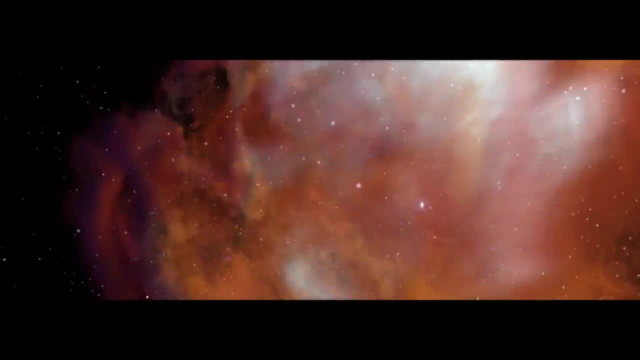 and its journey takes us way, way back. Four and a half billion years. The raw ingredients of Bennu and our Solar System originated in a stellar nursery, A vast cloud of hydrogen helium and dust. Our own Sun doesn't yet exist. 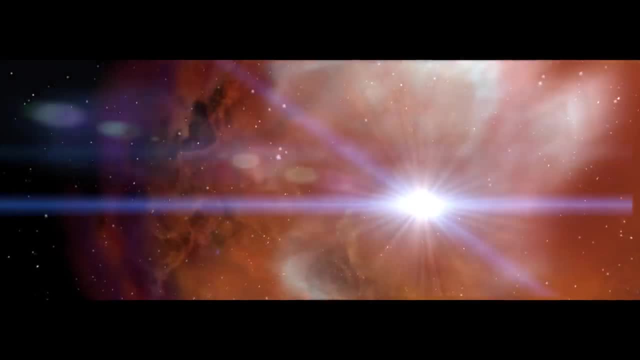 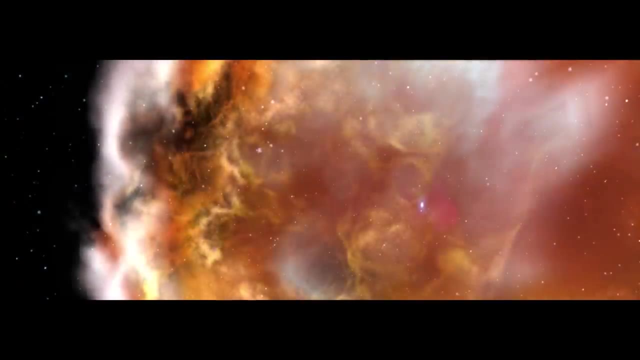 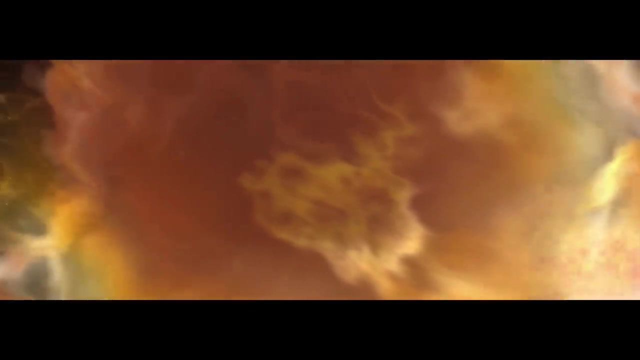 Nearby are hot stars like this one, Quickly burning up its fuel and destroying itself in a colossal explosion called a supernova. The explosion destabilizes our cloud, causing it to collapse In the geologic blink of an eye- a hundred thousand years. 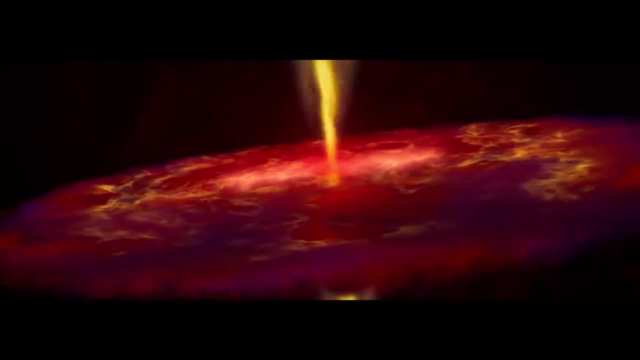 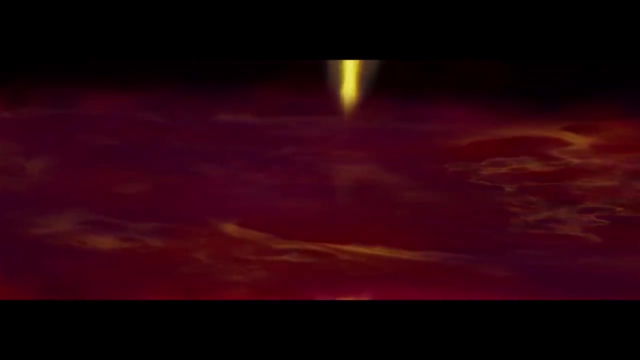 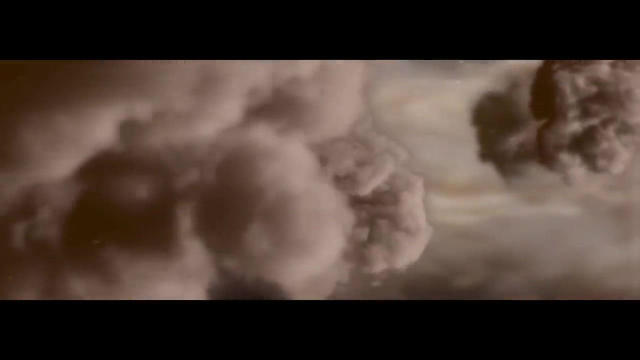 gravity and angular momentum flatten the cloud into a swirling disk In the center, where molecules crash together tightest. a protostar revs up to incredible pressures and temperatures. Deep within the disk, clumps of dust not much larger than a grain of wheat. 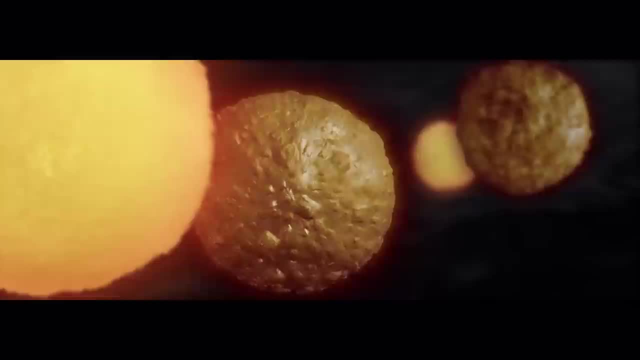 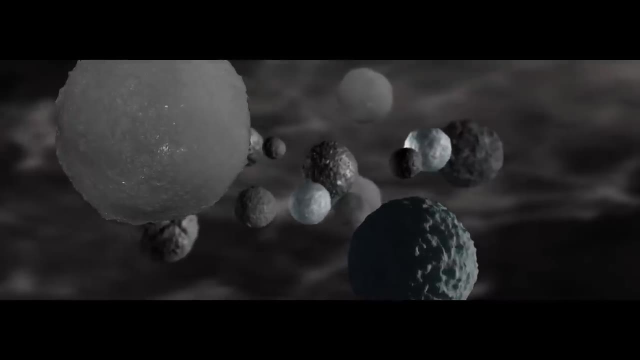 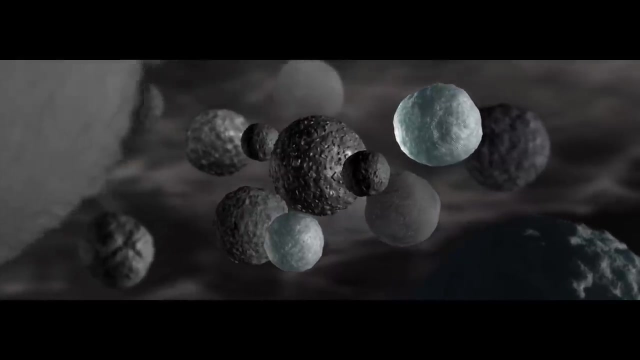 are flash-heated into droplets of molten rock called chondrules. The source of this heat remains a mystery. Chondrules are destined to become the building blocks of the Solar System. Coaxed by gravity and turbulence, the chondrules clump. 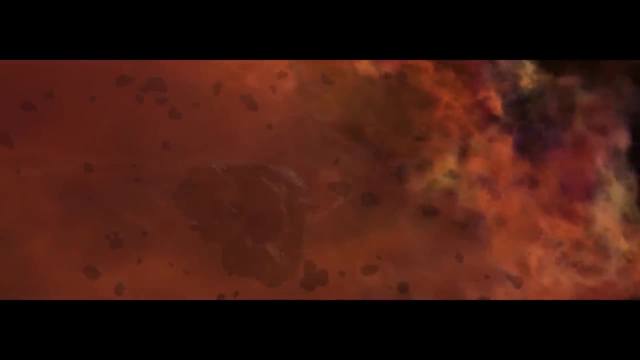 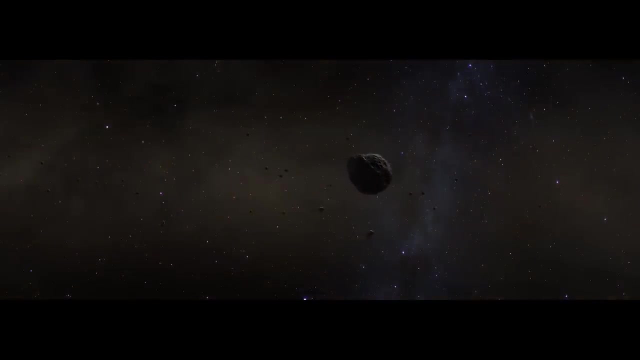 They grow into the first asteroids, into mountains, into planets. The asteroids are rubble, piles of rock, metal, ice and organics. This large asteroid is the parent body of Bennu, a protoplanet whose size we can only guess. 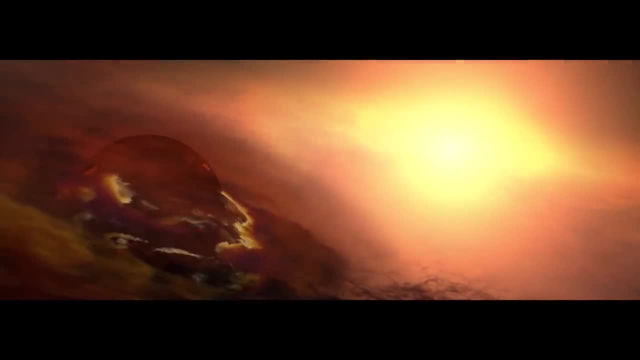 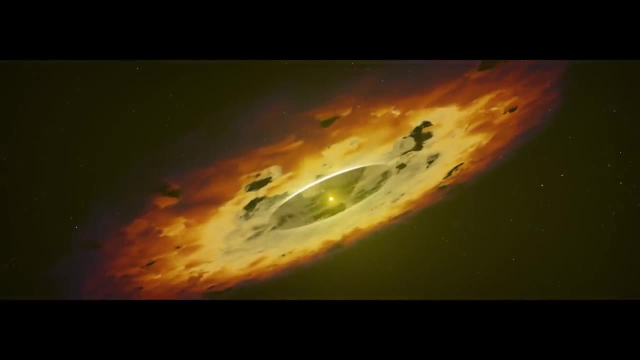 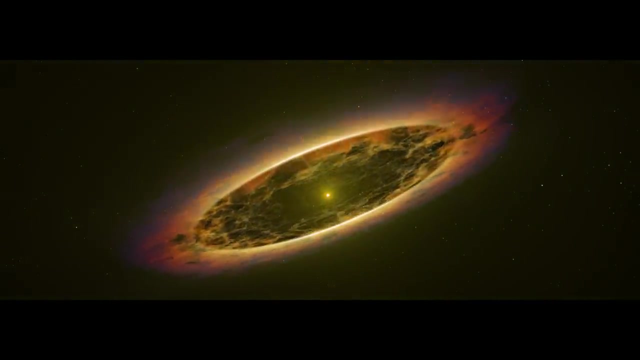 Closer to the protostar, a planet begins to form And then dawn in the Solar System. The protostar undergoes fusion and ignites, revealing our Sun. But the Solar System is far from finished. Jupiter most likely forms near its outer edge. 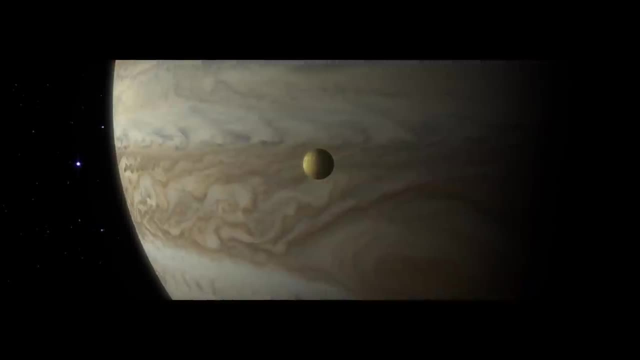 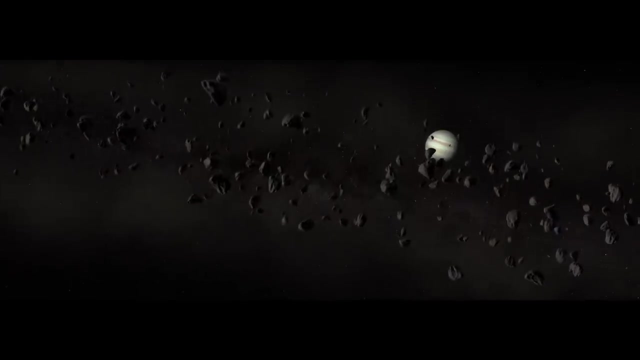 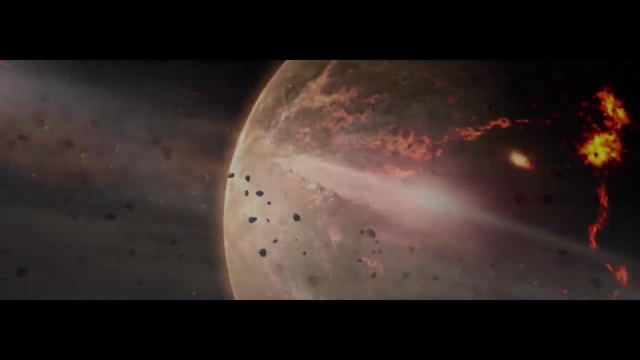 But just 500 million years after the Sun ignites, some believe that it slowly moves inward. Its massive gravity ripples the asteroid belt, disrupting countless asteroids and comets, flinging them toward the Sun. They rain down on the inner planets. 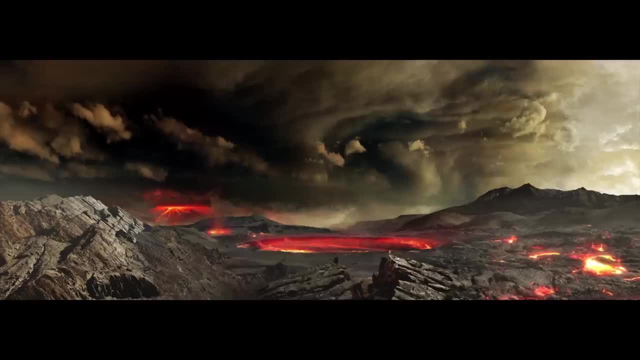 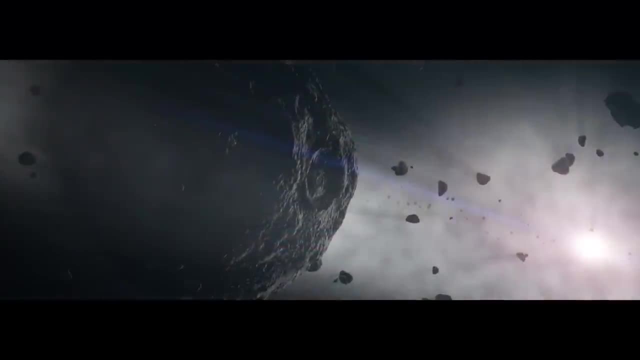 hammering and remelting large portions of their crust? Did these impacts also deliver organics and water, key ingredients for life Back in the asteroid belt? Bennu's parent body is lucky: It survives this period of heavy bombardment. The Solar System cools and calms. 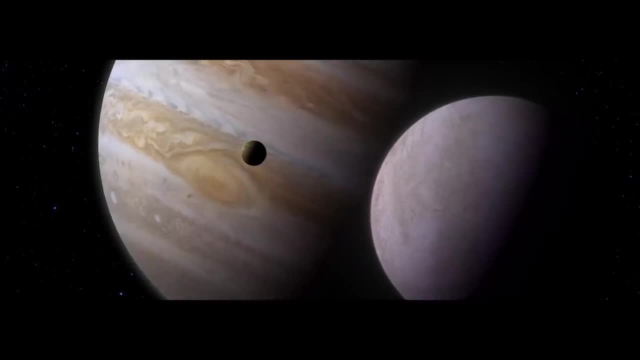 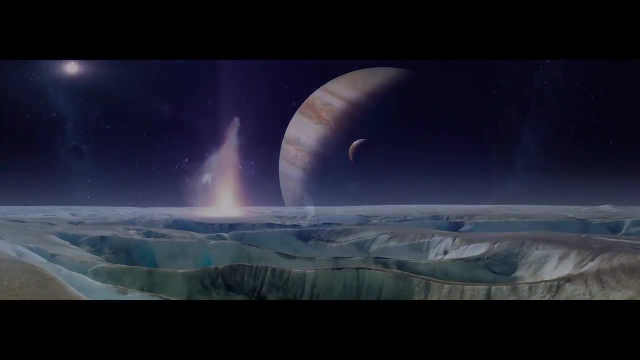 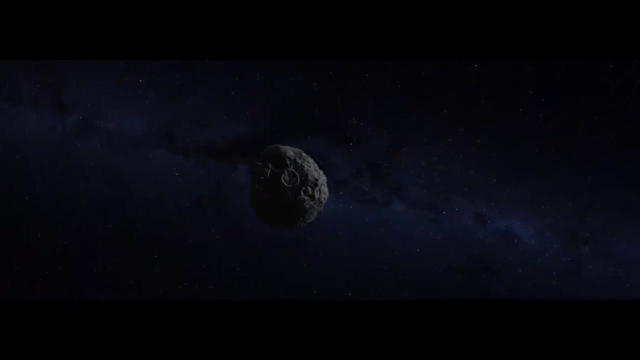 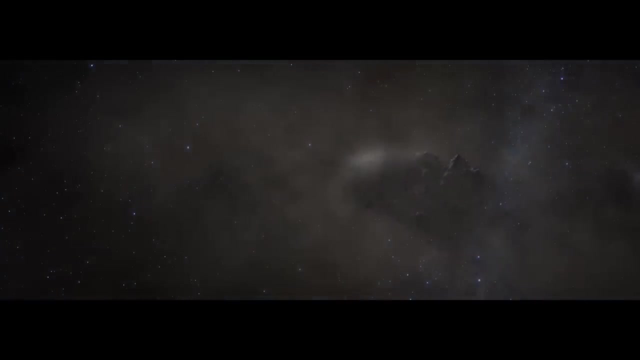 Jupiter and its many moons assume the orbits that we see today. Billions of years of quiet follow, More or less Then. a billion years ago, one theory suggests a collision shatters the protoplanet. Some of the debris loosely coalesces into a new, smaller body. 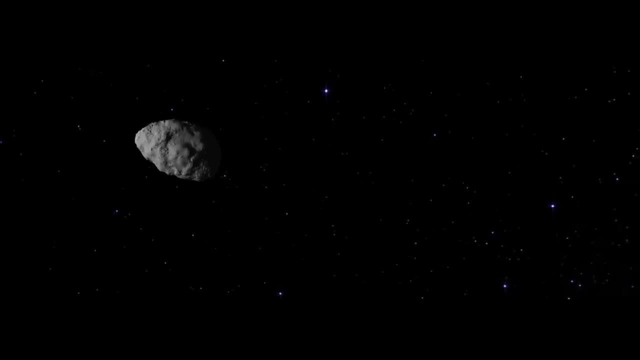 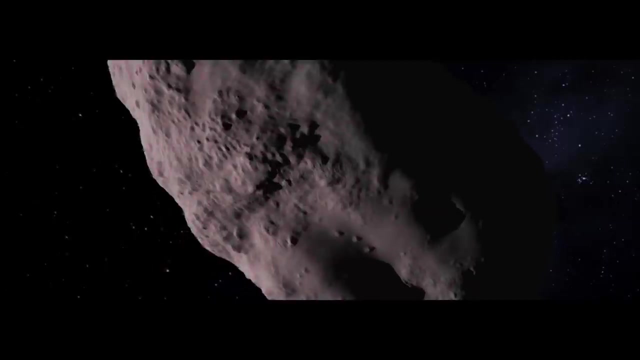 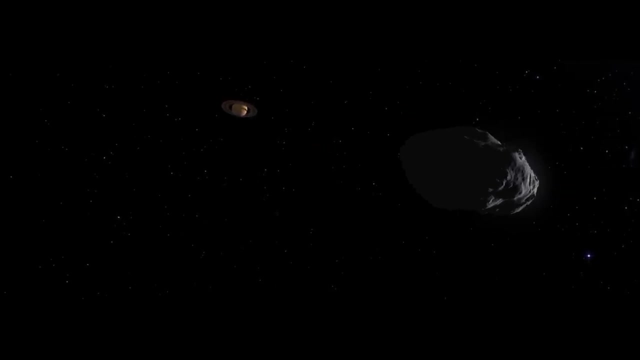 Bennu. But Bennu will not stay in place. Dull, non-reflective, it slowly migrates toward the Sun. Solar heating turns its warm side into a low-intensity thruster Through millions of years. Bennu's orbit gradually tightens. 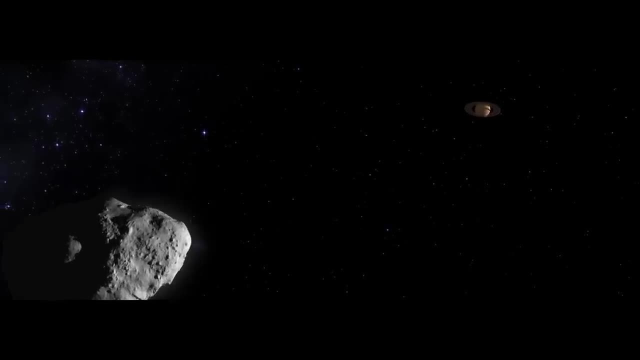 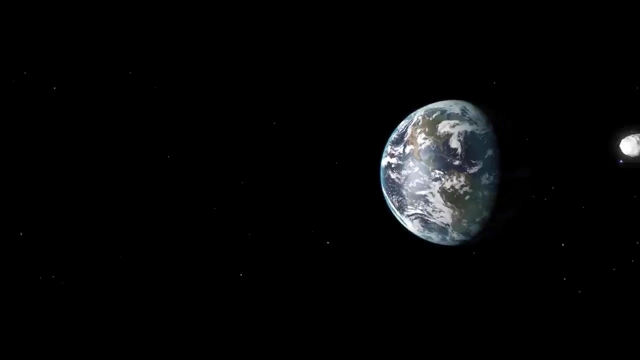 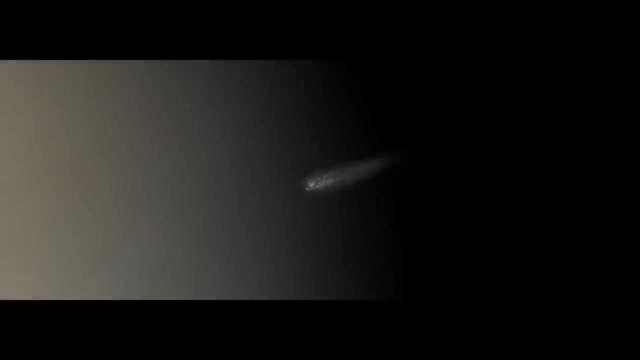 until it interacts with Saturn's gravity, altering its trajectory and hurling it into the inner Solar System. Close encounters with Earth and Venus follow. Their gravitational tugs may have repeatedly stretched and reformed Bennu, turning it inside out and pulling off loose material.